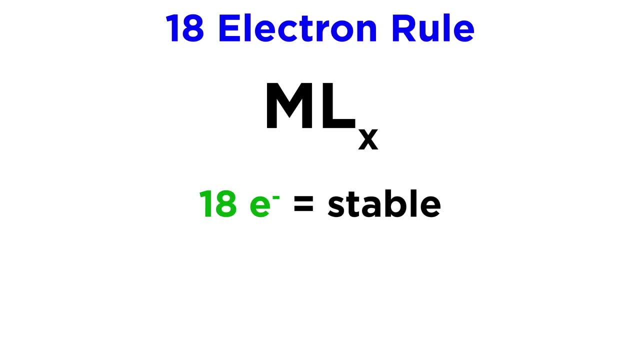 This will be a particularly stable situation thermodynamically, and complexes with fewer than eighteen electrons will often react in ways that lead to eighteen electron counts, while complexes with more than eighteen tend to be unstable and react in ways that reduce their electron count. This is more of a guideline than a firm rule. 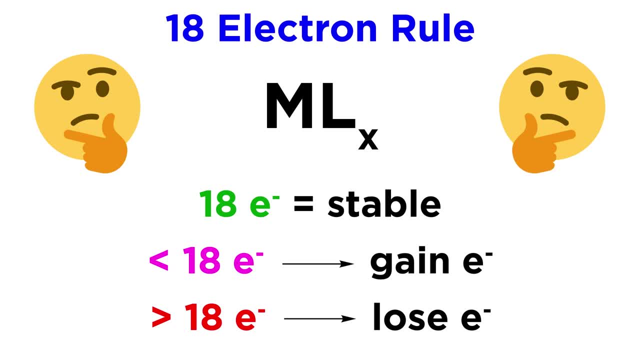 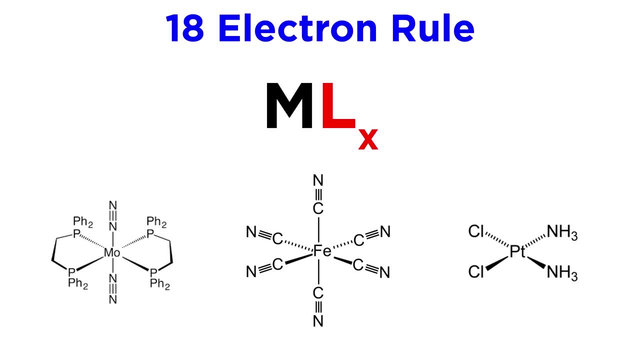 just as we quickly discovered when we learned the octet rule in general chemistry. but it is very useful nonetheless. We can now take what we learned in the past. few tutorials about common ligands and the number of electrons that they donate. in order to count these electrons for any complex 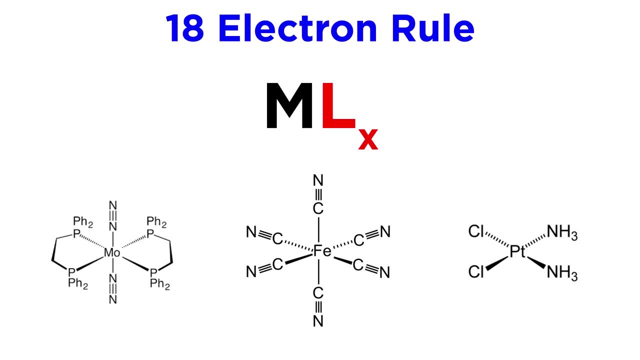 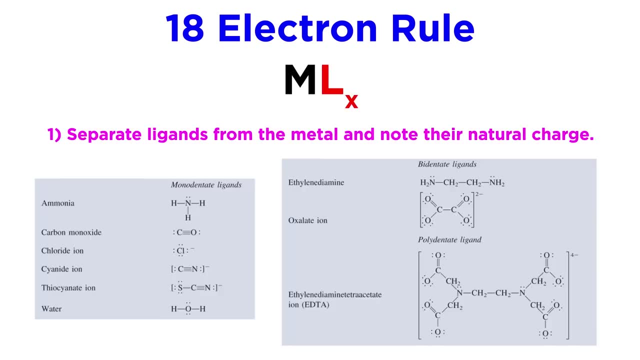 and determine whether the eighteen electron rule is being followed. Certain situations are trickier than others, but let's go ahead and learn a general algorithm that we can follow. First, we must separate each ligand from the metal and allow all ligands to exist with their natural 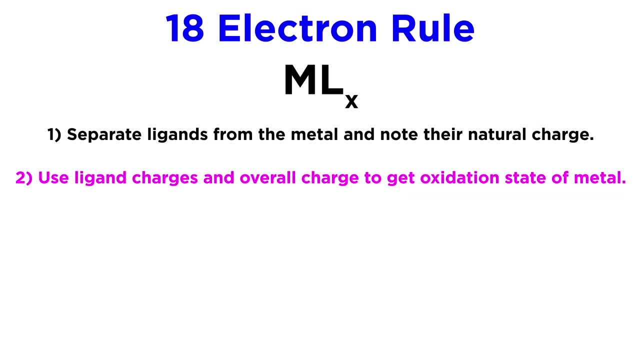 charge. Next, using the charges on the ligands and the overall charge on the complex, we can calculate the charge or oxidation state on the metal center. Because the charge on the metal plus the charges on the ligands should add up to the overall charge, we simply subtract the sum of the 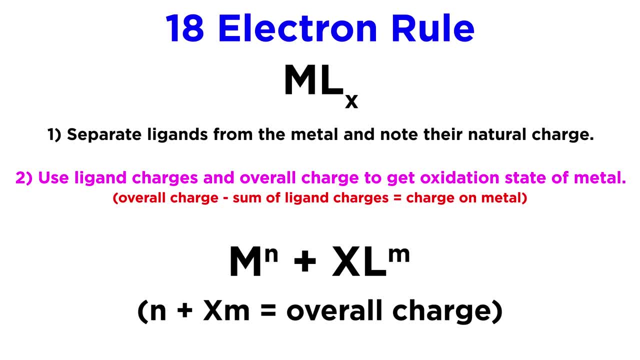 ligand charges from the overall charge to get the charge on the metal. Then, using this charge, we calculate the number of valence electrons on the metal. We simply take the number of valence electrons on the neutral metal atom and subtract the formal charge. Next we count the number of. 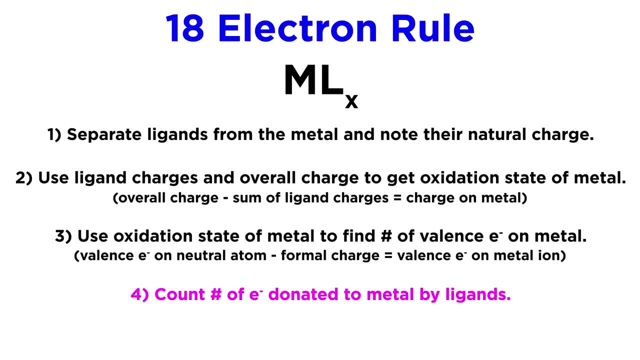 electrons that are being donated to the metal and add up the number of electrons that are being donated to the metal atom by the ligands. This isn't always immediately obvious, but we should be able to memorize electron counts for the common ligands quite easily, even the ones that are less. 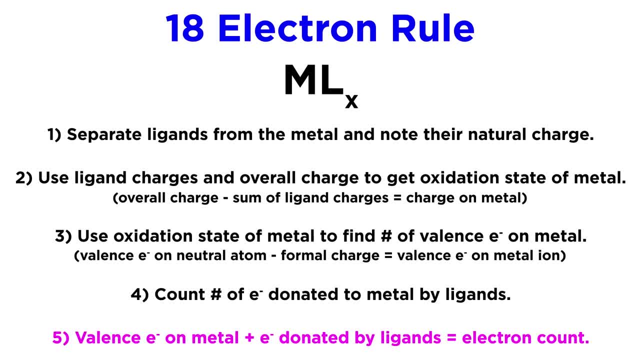 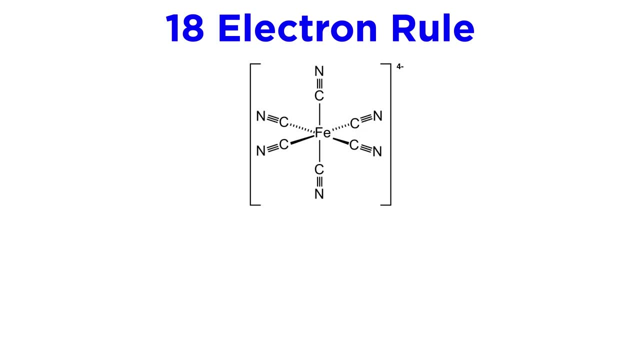 intuitive, so this shouldn't be a problem. Then add up the electrons on the metal and the electrons donated by the ligands. That's your electron count. This will make much more sense with an example, so let's try one. We have an iron atom and six cyanide ions. 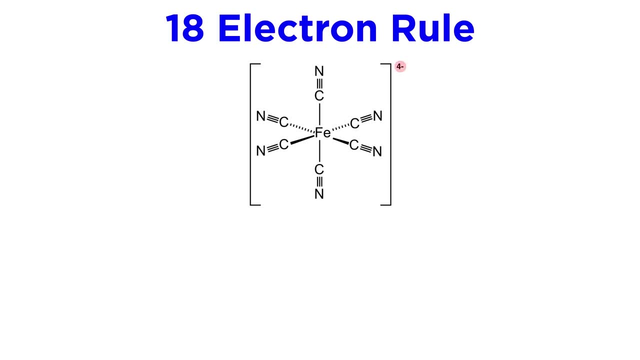 Which make a complex that has an overall charge of four minus. Let's go through the steps we just outlined. First, each cyanide ion is CN minus. like this, There is a triple bond between the atoms and a lone pair on each, which leaves carbon with a negative charge. There are six of these. 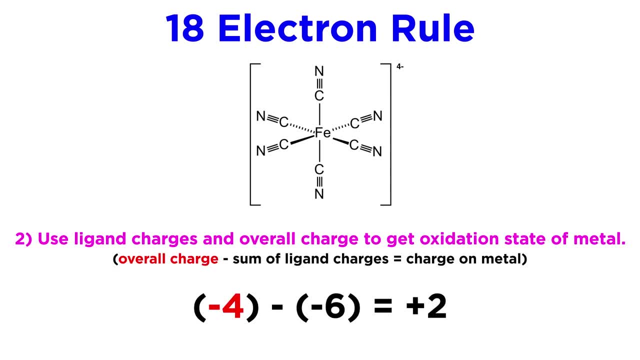 for a total of six minus and the overall charge is four minus, which means that the iron atom must have a charge of two plus, because two plus negative, two minus four minus, four minus two minus of six equals negative four. Now a neutral iron atom has an electron configuration ending. 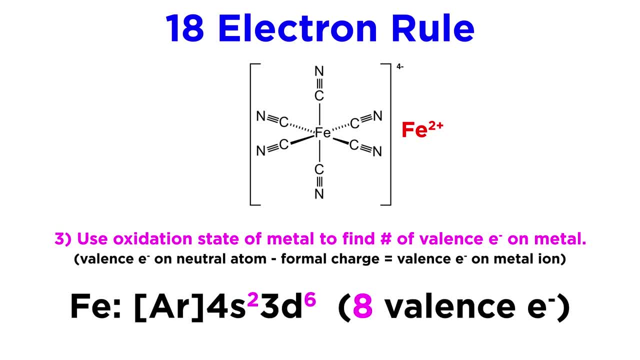 in 4s2 3d6, so it has eight valence electrons. This means that the two plus cation must have only six valence electrons, which happen to be the 6d electrons. So iron contributes six electrons to the total count. Each cyanide ion contributes two electrons, the two in 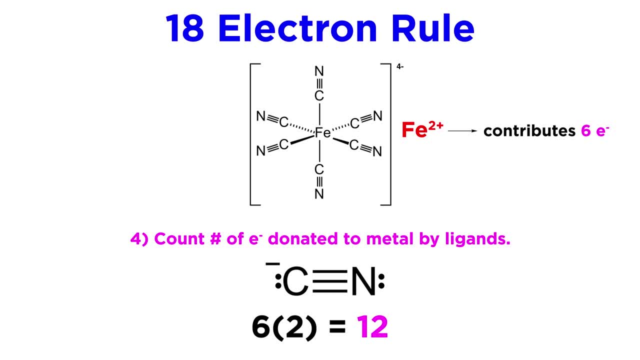 the lone pair on carbon, so that is a total of twelve from the cyanide ions. Six plus twelve is eighteen, so this complex does satisfy the eighteen electron rule and should be expected to be quite stable. Now, this one was pretty easy, but don't forget that we 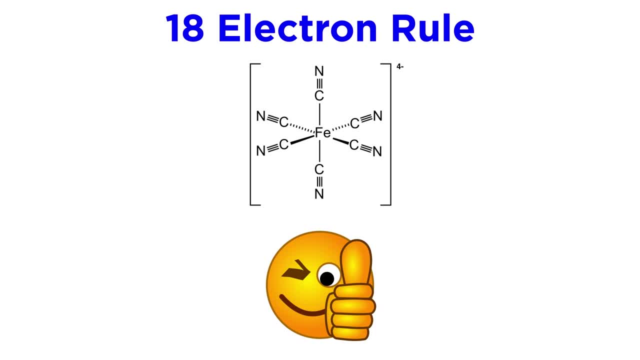 have all those polydentate and polyhapto ligands, So this can get a little trickier. Let's try this one Here. we have a tungsten center, we have a cyclopentadienyl anion, three trimethylphosphenes and two chlorides, with an overall charge of 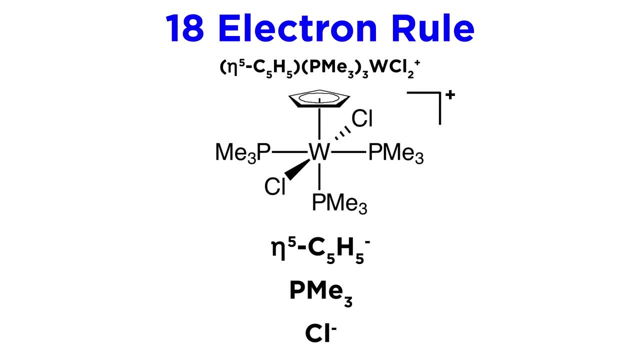 one plus. So let's go ahead and separate the ligands from the metal. This is the first place where mistakes can be made, as we need to know the charges on these ligands, even though they aren't shown explicitly in the formula. We must know that the cyclopentadienyl 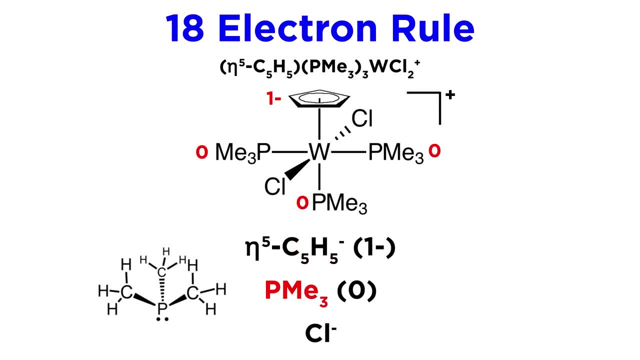 ligand is an anion. it has a one minus charge. The phosphenes are neutral- that makes sense from simple Lewis diagrams- And the chloride ligands have a negative charge as well. So adding up the charges on the ligands we get a total of three minus The charge on the. 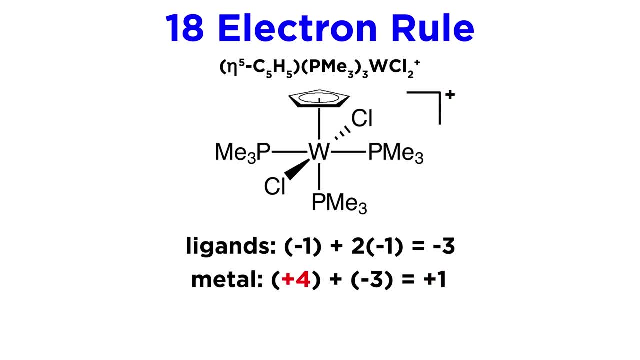 complex is one plus, so the oxidation state on tungsten must be plus four, since four plus negative three equals one. Now tungsten has an electron configuration ending in 6s2, 5d4,, so it has six valence electrons. 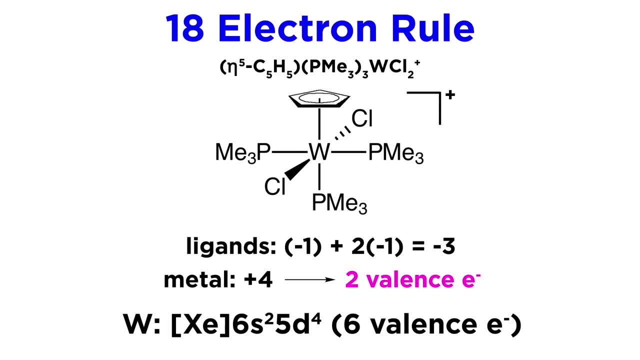 Losing four electrons therefore leaves us with only two. Now let's see how many electrons the ligands are contributing. The cyclopentadienyl anion donates three pairs of electrons, so it donates six electrons total. This one is very important to remember. The others are: 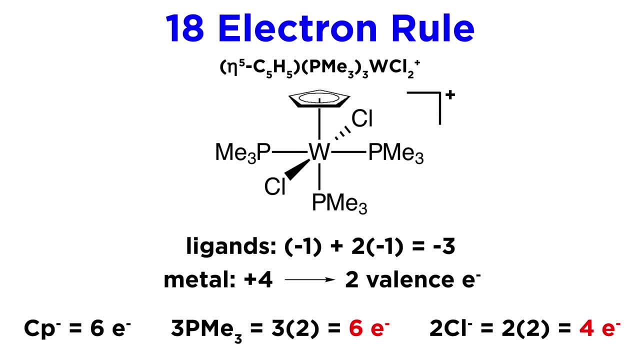 more obvious, the phosphenes and chlorides. So let's see how many electrons the ligands are contributing. The cyclopentadienyl anion donates three pairs of electrons, so it donates two electrons each. So that's six plus six plus four for a total of sixteen electrons. 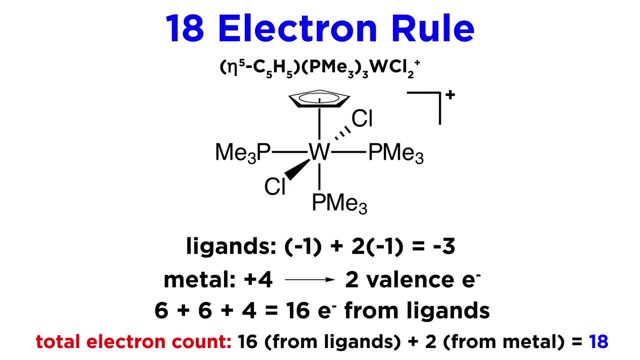 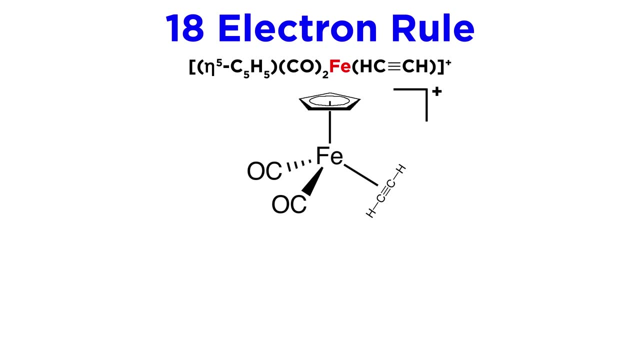 from the ligands, Add the two from the metal atom and we get eighteen. so this complex satisfies the eighteen electron rule and should be quite stable. Now let's try something slightly different. Here is a complex with an iron center surrounded by a cyclopentadienyl. 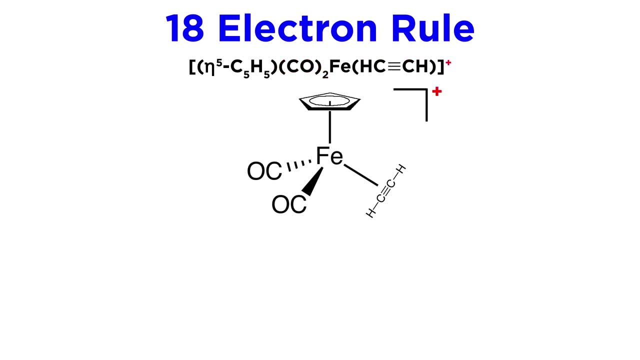 anion: two carbonyls and an alkyne, with a one plus charge. Let's try and predict whether the alkyne is a two electron or four electron donor in this complex. So first let's separate the ligands, those being the Cp- two neutral carbonyls and the alkyne. That's. 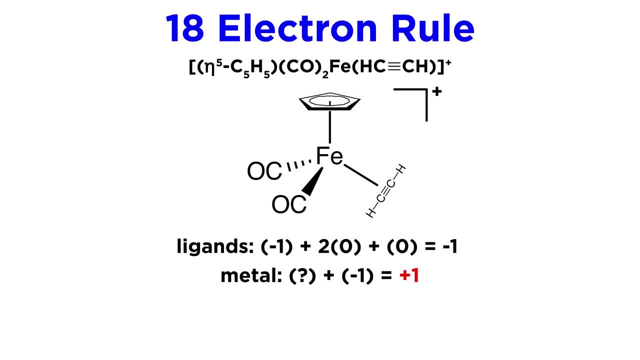 a total charge of one minus for the ligands and we have to get to one plus overall. so the metal must be in the plus two oxidation state. Since iron has eight valence electrons, a cation in the plus two oxidation state must. 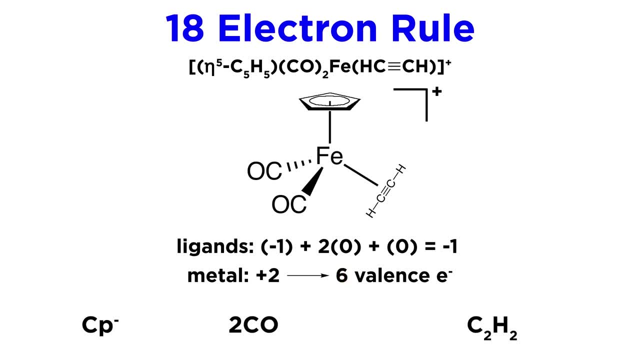 have six electrons. Now back to the ligands. This cyclic ligand contributes six electrons, Each carbonyl contributes two and then once again, the alkyne contributes either two or four. Now let's take the six from the iron, plus six from this ligand, plus four from 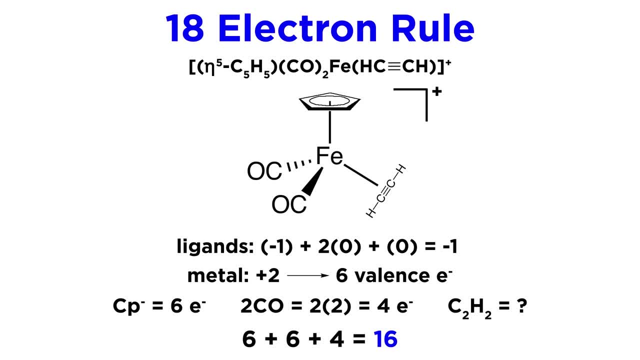 the carbonyls. and that gets us all the four. So the six roughly is equal to the halogen. welcome to our activation At Kong fra dr alla way to 16.. Two more electrons would get us to 18. This means that due to the 18-electron rule, 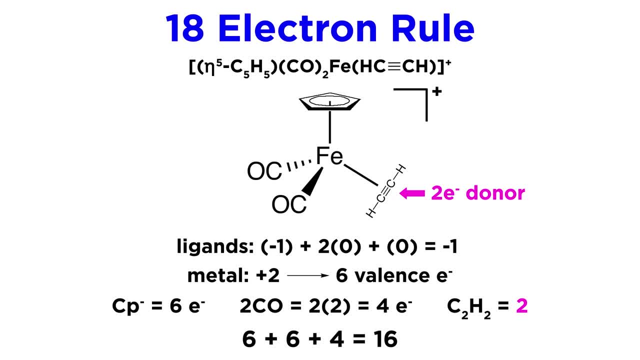 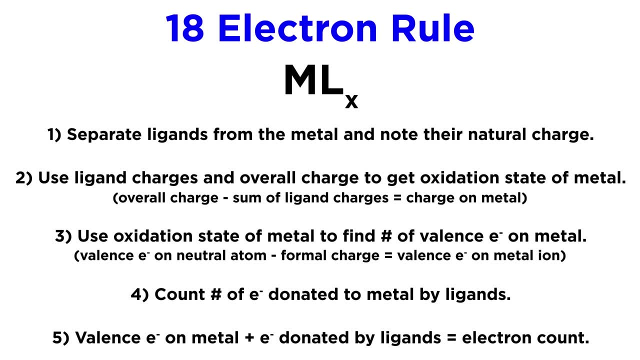 the alkyne is likely acting as a two-electron donor in this complex. So that gives us an introduction to the 18-electron rule, which will be very important for understanding all the transition metal complexes we will soon be learning about. Remember, all we have to do is separate the ligands, use their charges and the overall charge. 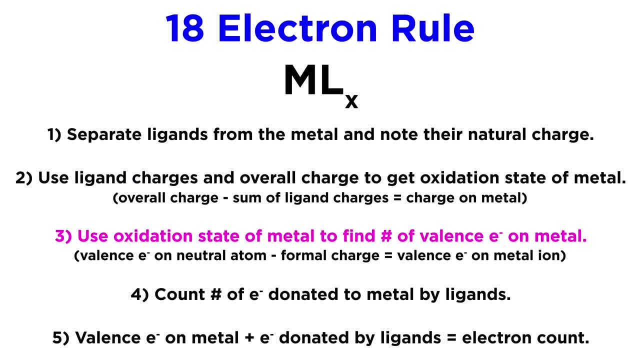 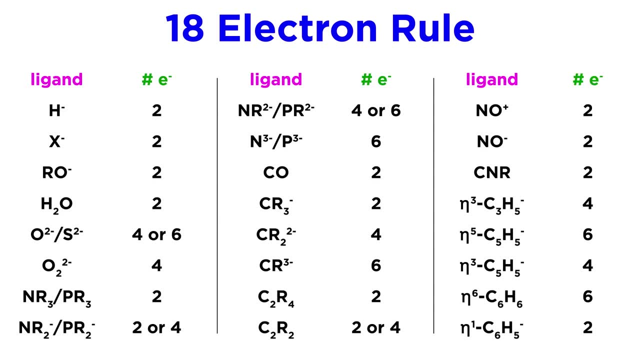 to get the charge on the metal. use that to determine the number of valence electrons possessed by the metal and then add that to the number of electrons contributed by the ligands. If we get to 18, the complex is stable. We may want to memorize this chart which tells us the 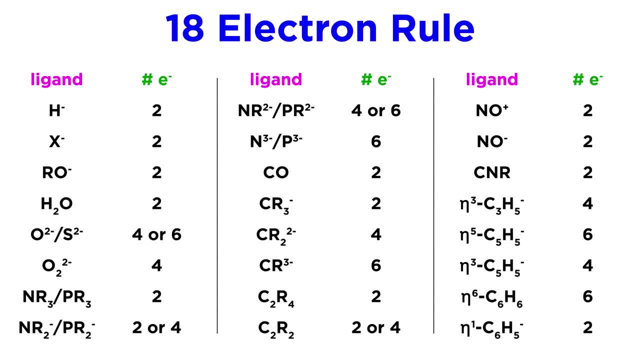 number of electrons contributed by the most common ligands and their charges, as some of them are very similar to the number of electrons in the ligands. and the number of electrons in the ligands are not as intuitive, although many of them are very easy to remember. It is also best to 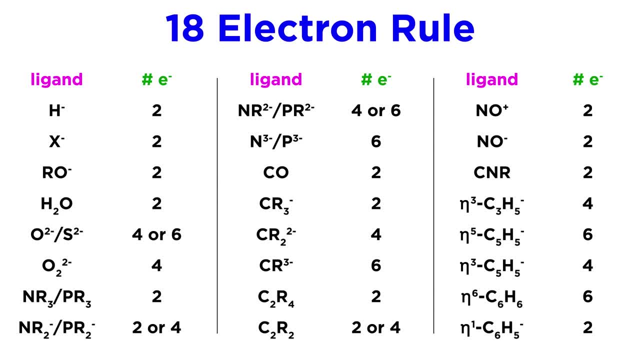 bear in mind that there are alternative counting schemes. The charges and electron counts covered in this tutorial are the most commonly used, but in the end they are merely a convention. Other sources may consider alkylidines to be neutral rather than 2- and alkylidines 1- rather than. 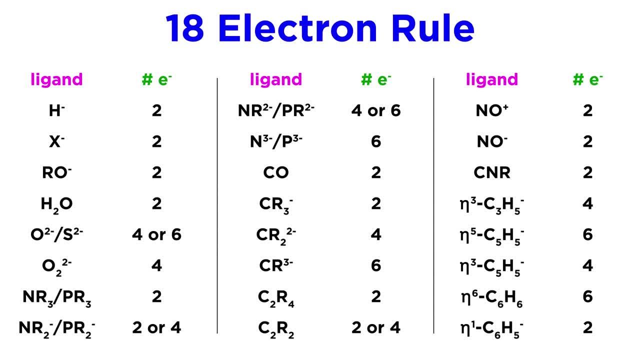 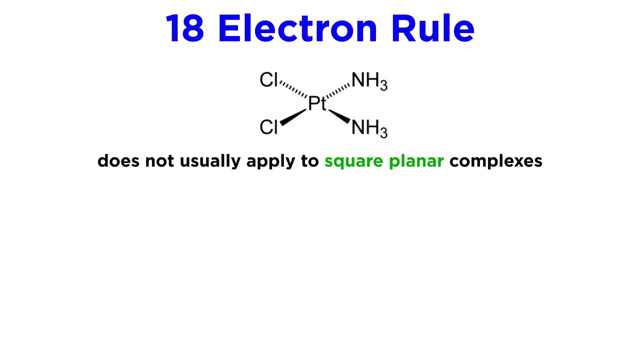 3-. This is simply another convention and the total count will still be 18, so if you encounter a discrepancy with other sources, take note of the difference in the approach as best you can. We also have to mention some exceptions. The 18 electron rule does not usually apply to. 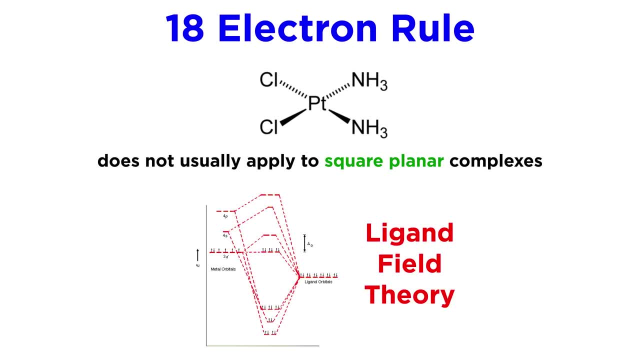 square planar complexes. We will come to understand why just a bit later, when we investigate ligand field theory, but for now just know that square planar complexes will be most stable with a 16 electron count. This is common for complexes with platinum 2 and palladium 2.. 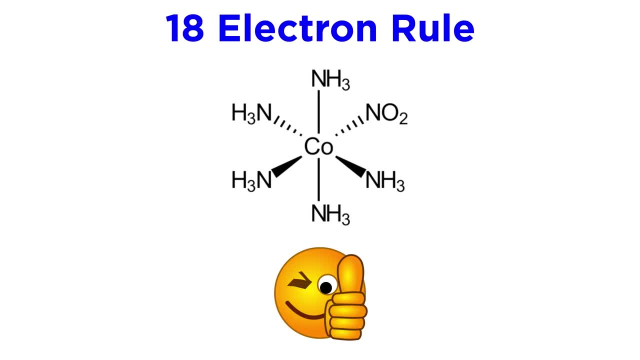 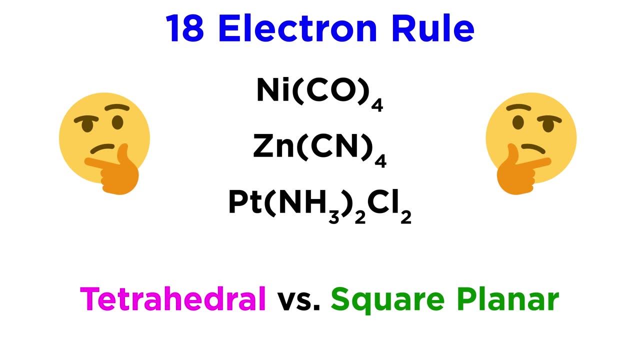 So when you see an octahedral complex, don't worry about it. you know, 18 electrons is the goal. If you see a formula for a complex with four monodentate ligands, however, you will have to figure out first whether the complex is tetrahedral or square planar in order to make an assessment. 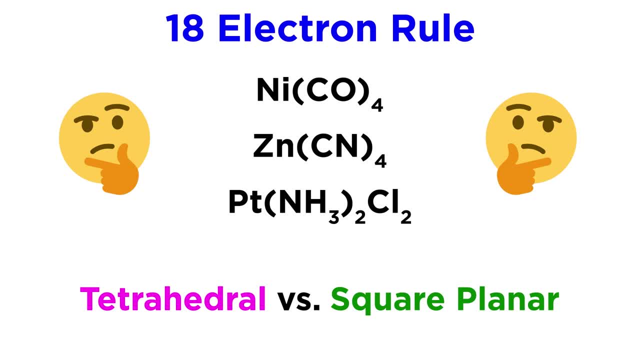 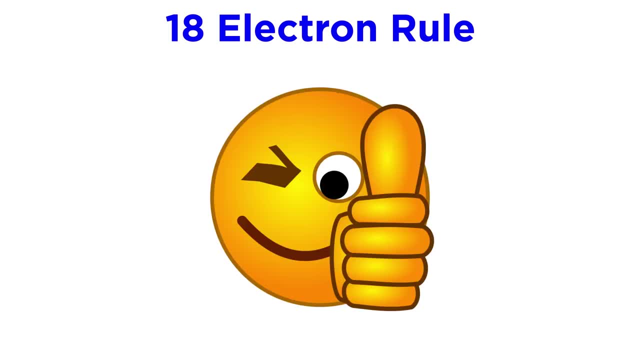 regarding electron count. But don't worry, we aren't there quite yet. we just had to mention this caveat right now to be thorough. For the moment, let's just continue and get a little more practice with the 18 electron rule. For now, let's just continue and get a little more practice with the 18 electron count. 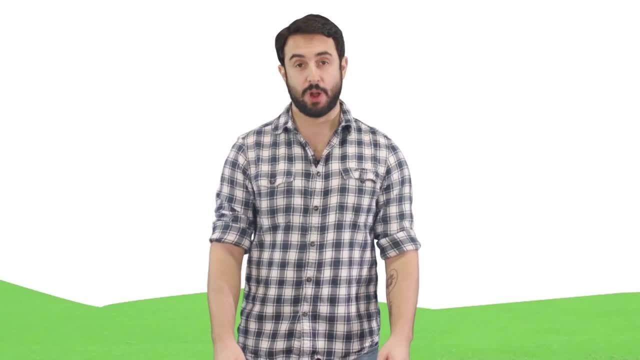 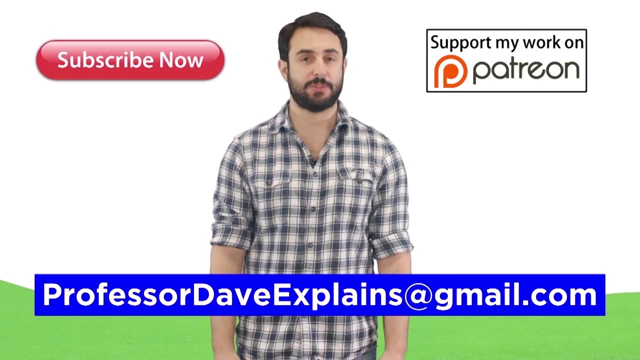 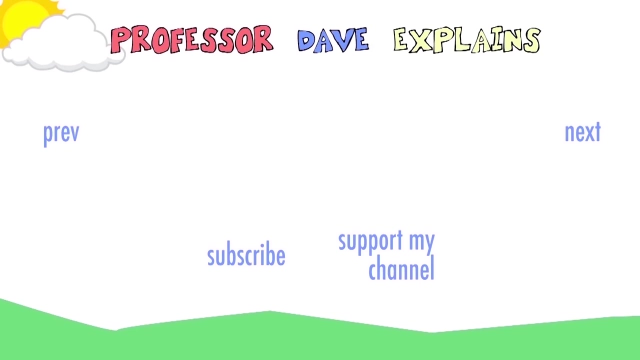 For now, let's just continue and get a little more practice with the 18 electron rule. For now, let's just continue and get a little more practice with the 18 electron count.